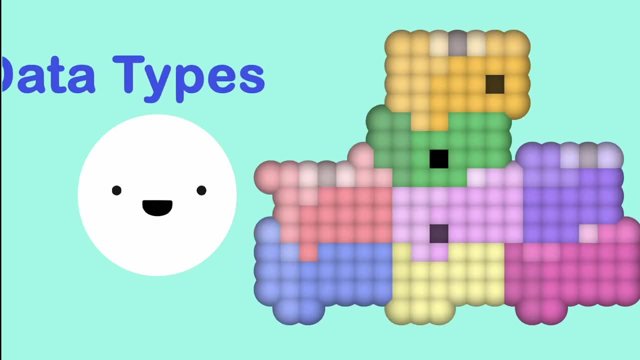 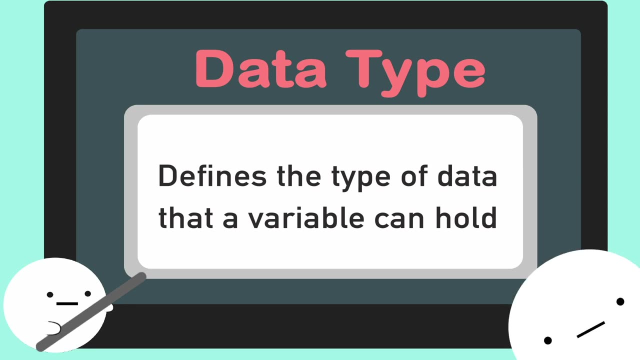 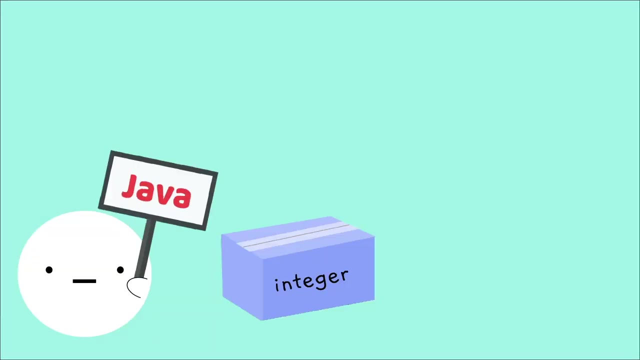 of categories. In programming these things would be known as data types. A variable's data type determines the type of data. For example, the language Java has many different data types, including integer, character, byte strings, short, long, boolean, double and float. We won't go into detail of exactly. 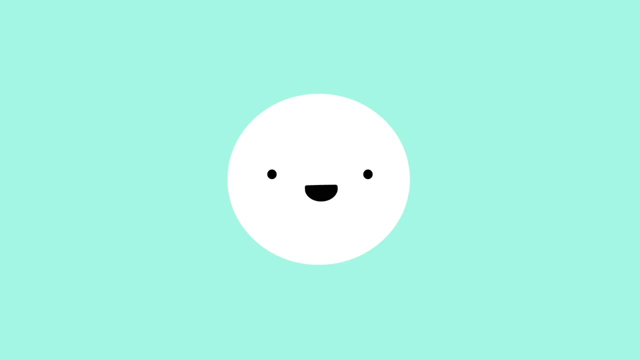 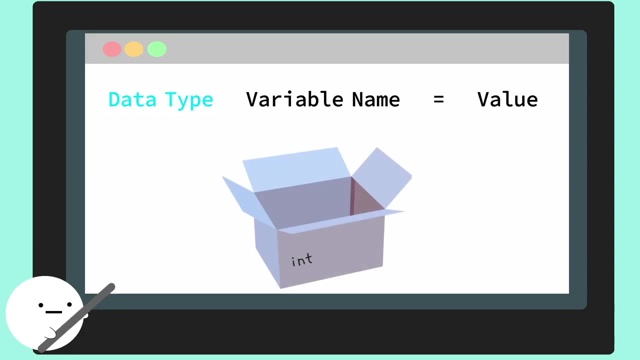 what these data types do here, but we'll talk about them in another video. Now let's go ahead and see how we write a variable. Before using a variable, you gotta create it. Creating a variable is known as declaring a variable. When coding a variable, you'll generally first declare its data type, then its name. 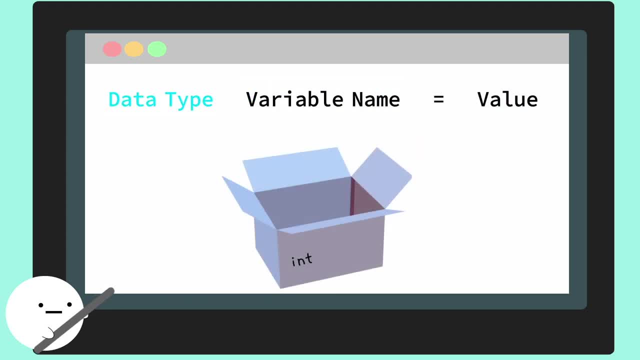 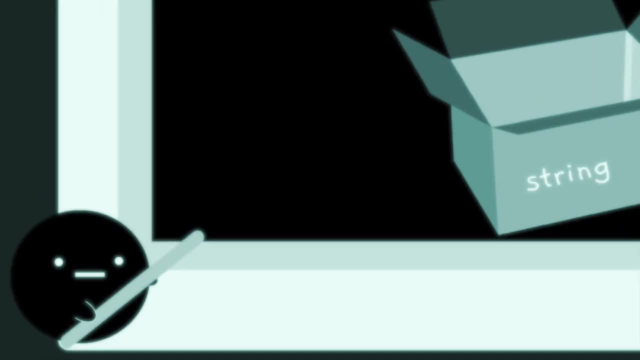 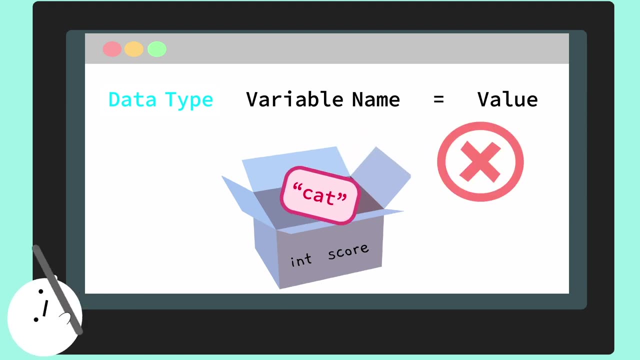 then assign it a value. First you declare the variable's data type to determine what you want to store in this variable. Maybe you want to make it store a number or even a word, But remember you can only store values of that variable's data type, so don't go storing words inside of integer boxes. 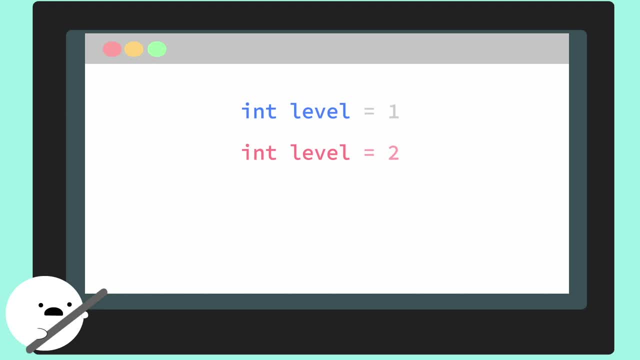 Also, you only need to specify a variable's data type the first time you declare it, so you don't need to state that your variable is an integer or a string every time you want to reuse it Next. you would give your variable a name. When giving your variables names, it's important. 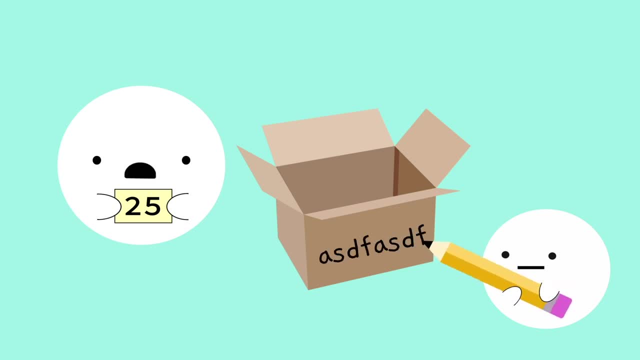 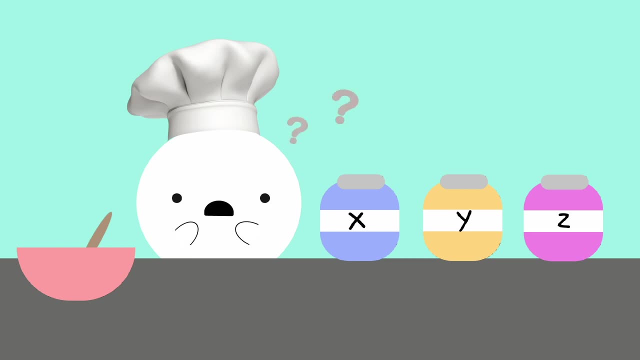 that you name them something meaningful rather than something undescriptive or random. It's like if you were baking a cake and had three jars labeled X, Y and Z. You wouldn't know which one's your flour, which one's your sugar and which one's grandma's ashes. 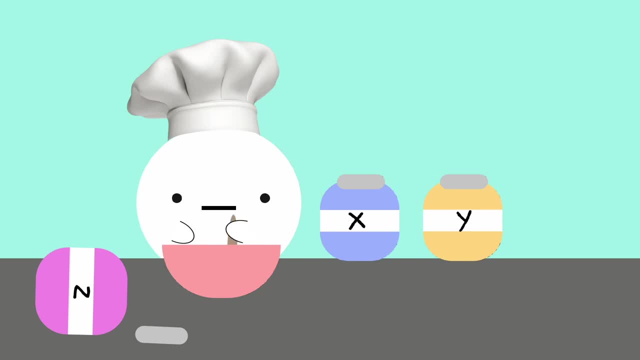 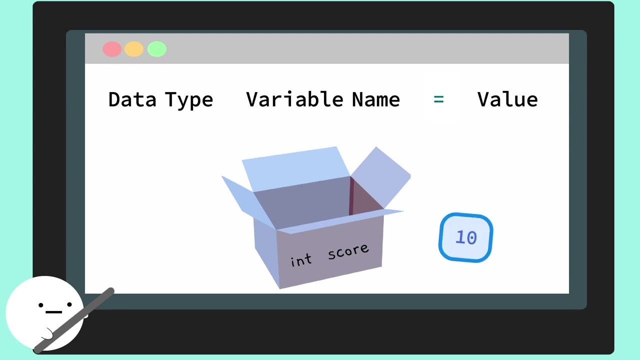 Mixing up your variable names, or in this case jars, could lead to many issues. Oh, no More grandma-flavored cake. So using meaningful names will help you easily identify the use of that variable later on in your program. After giving it a name, you could then assign it a value. 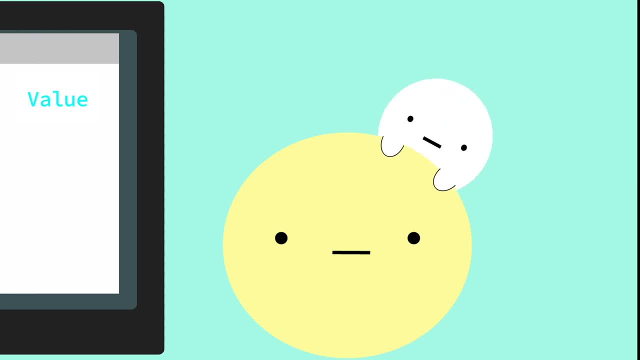 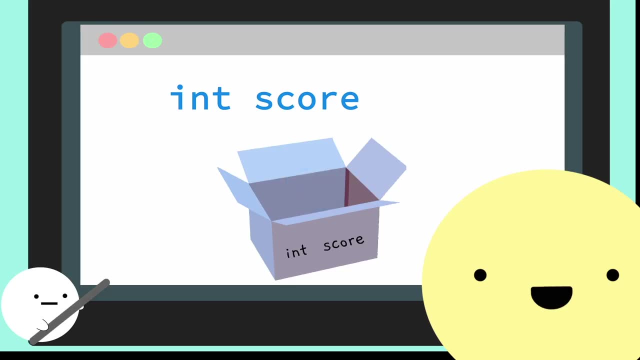 Do we have to assign it a value? No, Kevin, If you want, you can declare your variable without a value. It would just be an empty box. in that case, Once you declare your variable, there are a lot of ways to use it.